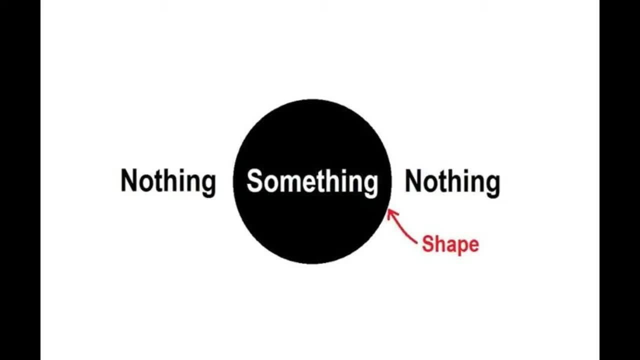 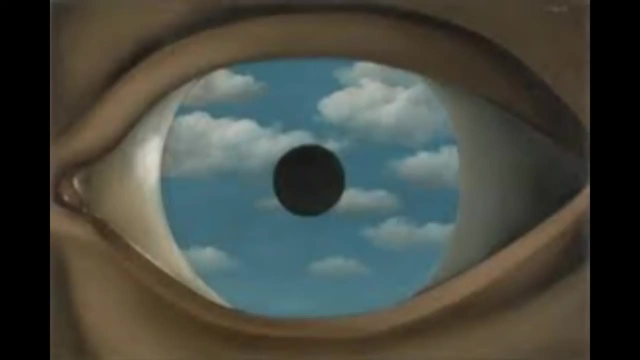 There is literally nothing to study at all. So I looked up the Proto-Indo-European root word for the verb to see which is where visualization comes from, And I thought it was interesting to find that many languages use this verb as a root word for other derivative concepts. 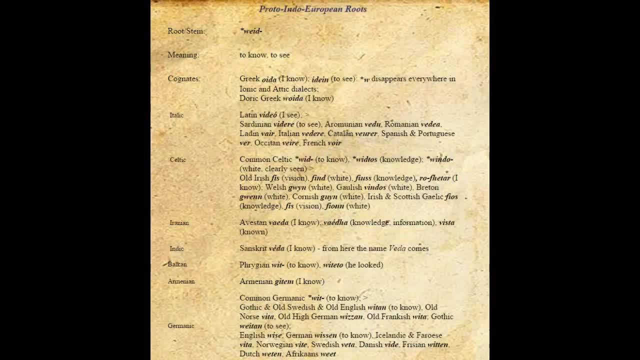 For example in Dork Greek means, I know, which is all derived from the Proto-Indo-European root word of wide, which is to see. Common Celtic is to know. is knowledge In Iranian, is knowledge or information? 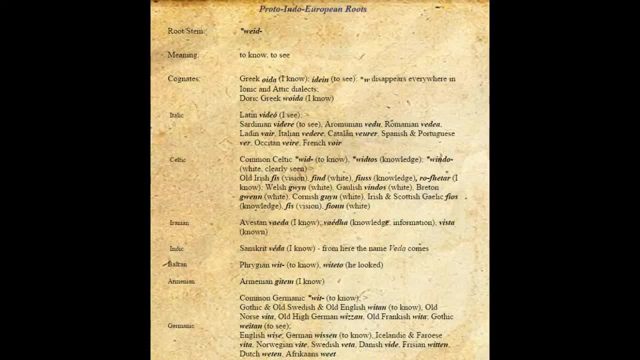 In Sanskrit means I know, which is where the name Vedas comes from, Which are the name of the ancient Hindu scriptures. In common Germanic means to know, means to see, means news in Russian. 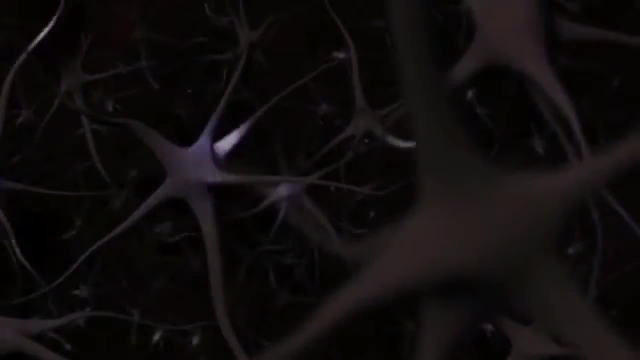 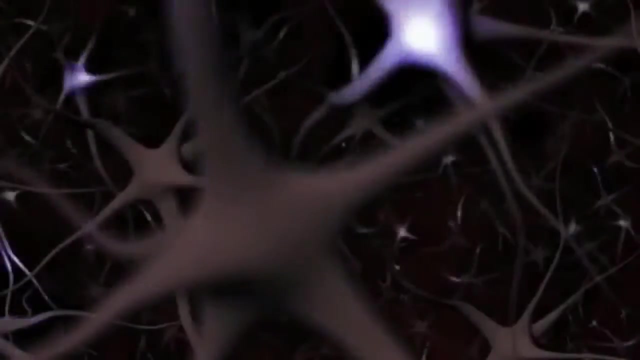 So not only did knowledge terms spawn from the idea of to see, but so did concepts of information and knowledge, But so did concepts of information and knowledge, But so did concepts of information and knowledge And news. 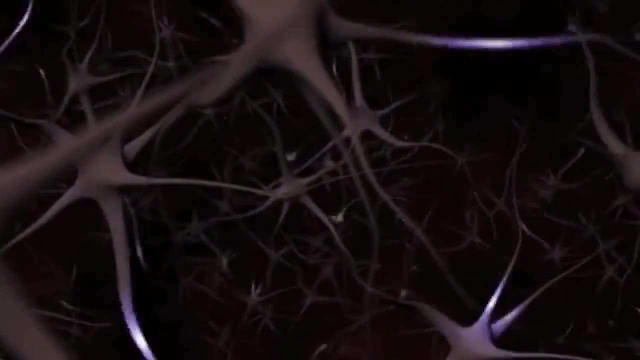 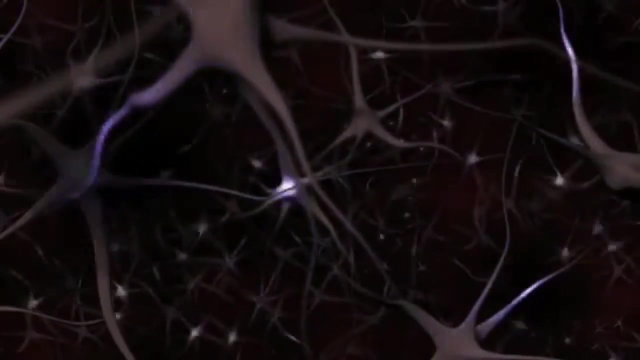 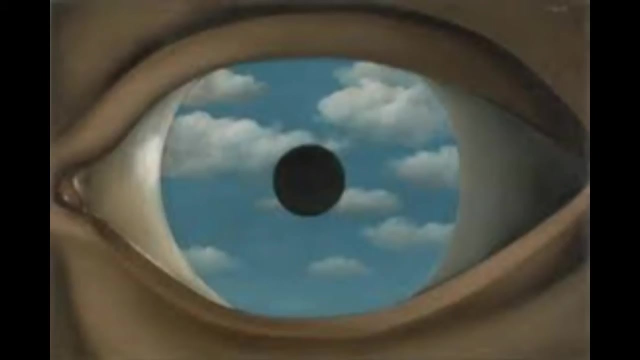 Now some people think that a good explanation for this is just that the word I know means I have seen. But I disagree with this explanation. I think that a more rational explanation is that knowledge is very commonly equated amongst most layman, most common speakers. 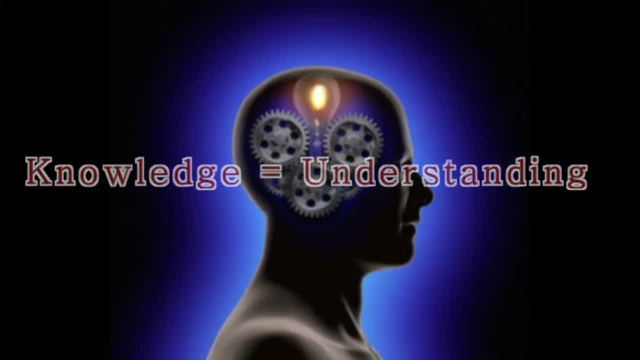 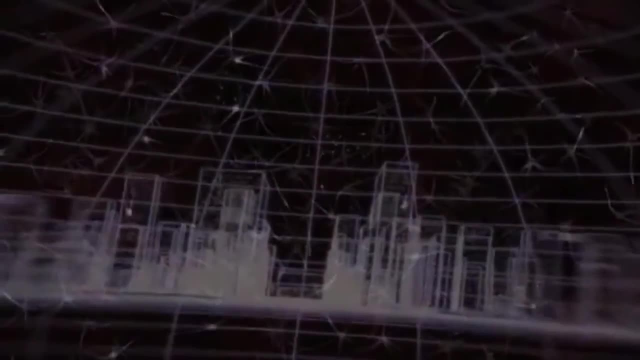 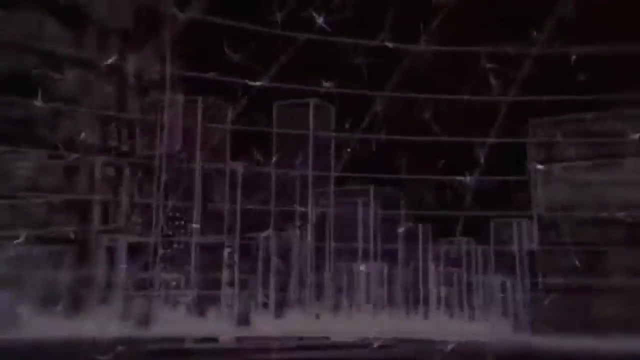 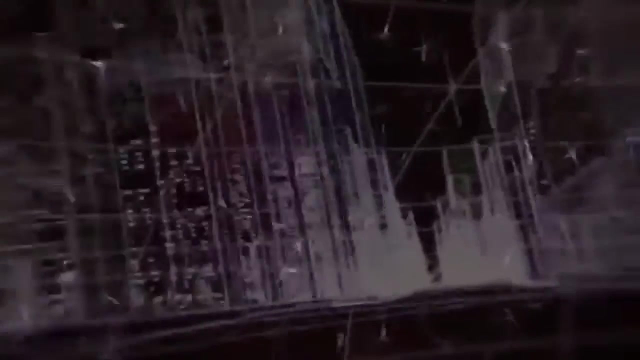 with understanding. We'll say: I know how that works or I know what caused that. It's equated with understanding and used synonymously with understanding which doesn't require you to see something directly. For instance, I can understand that the earth. 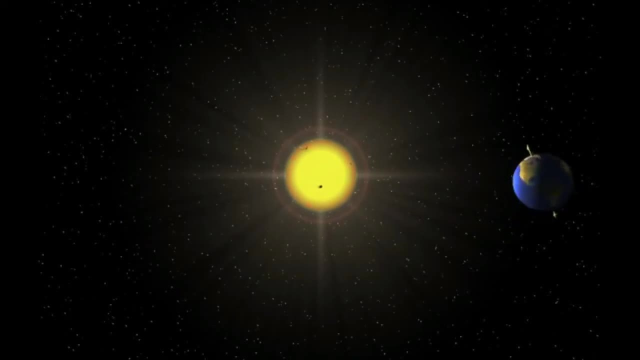 travels around the sun instead of the sun traveling around the earth. by just imagining it in my brain alone. I don't need to go outside of the atmosphere and look at earth from a distance and watch the earth travel around the sun. All I have to do is imagine it and I can understand. 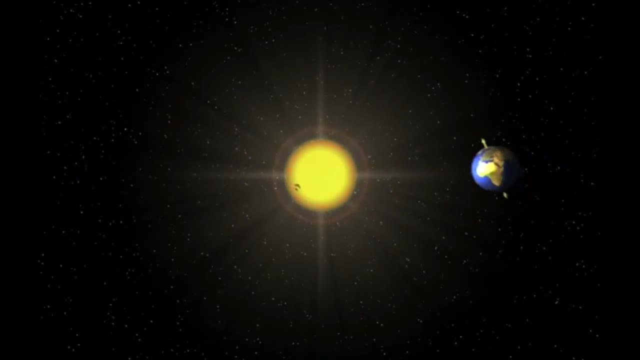 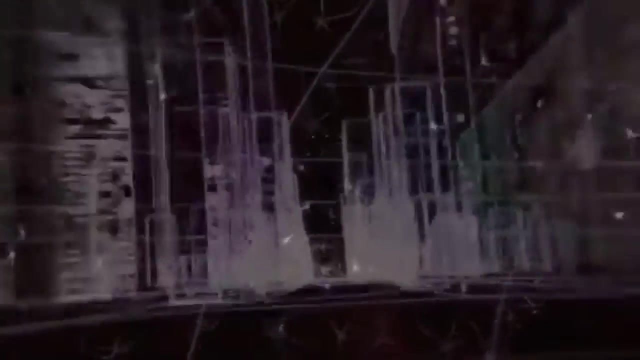 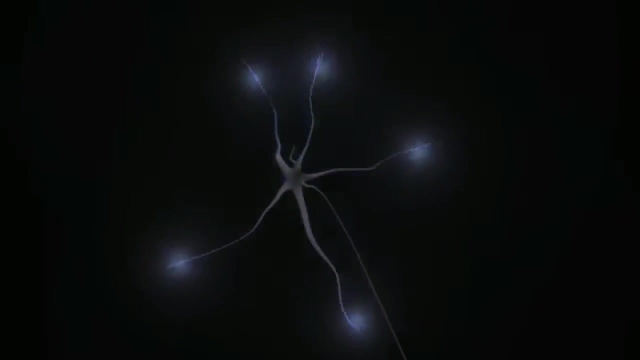 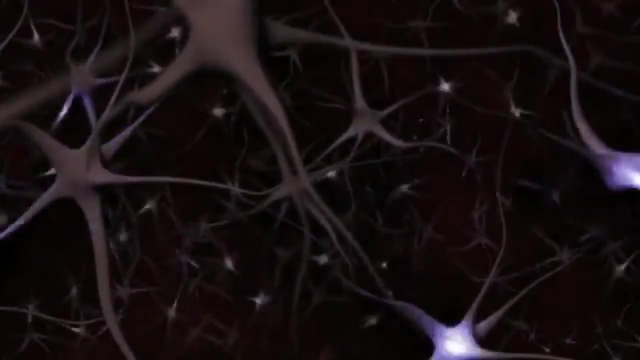 how that's possible. So what I think that the connection of knowledge between the earth and the sun is is that the earth travels around the sun, Which really is to say understanding and information and news. The connection of those to the concept of to see indicates some intuitive grasp that we used to have on the dependency of 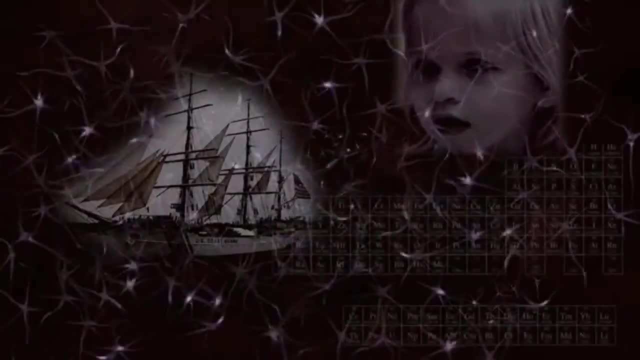 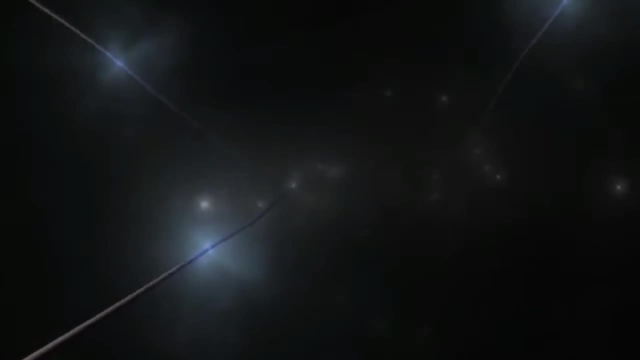 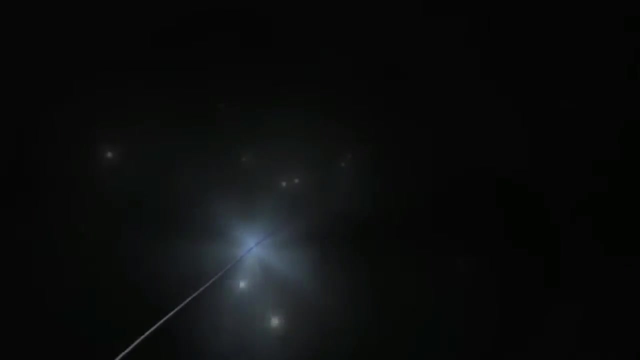 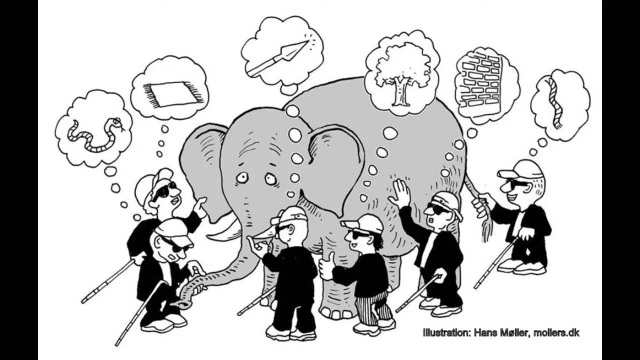 thought upon the visualization of objects. Visualization is not just important, but 100% crucial, because this is the only way to communicate what is on your mind objectively. It reminds me of the story of the three blind men describing their experience of an elephant. Each blind man feels a different part of the object and, based on their verbal descriptions to each other, each blind man comes to a completely different conclusion about what the object is. However, if each of these blind men was presented the object as a whole, say a mini-object, then it would be a completely different conclusion about what the object is. 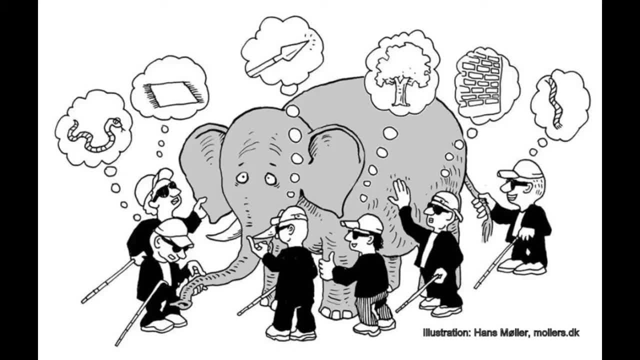 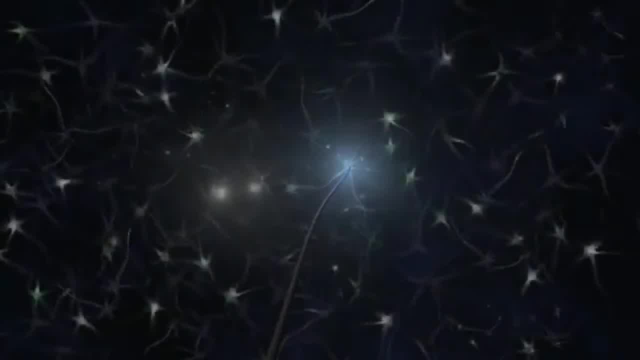 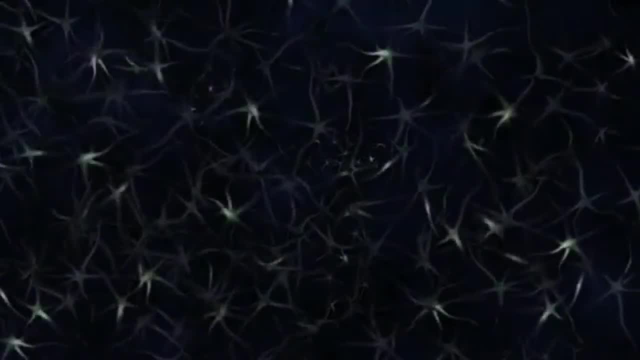 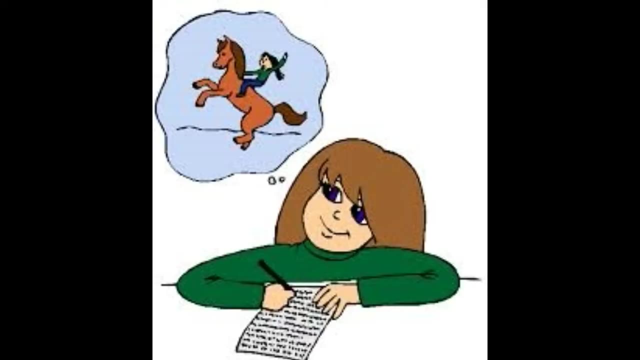 The idea is that the blind man is a miniature scale model, Instead of being allowed to feel only a small part of the elephant. then the confusion would be instantly resolved, because the entire entity could then be visualized, even to a blind man. Descriptions are only ever useful when referring to a physically present object. Only then can we unambiguously resolve the referent of the object. 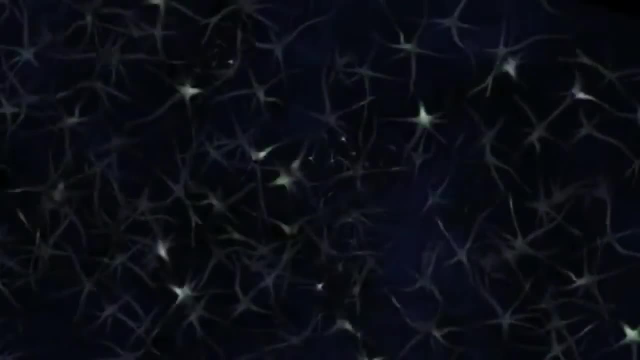 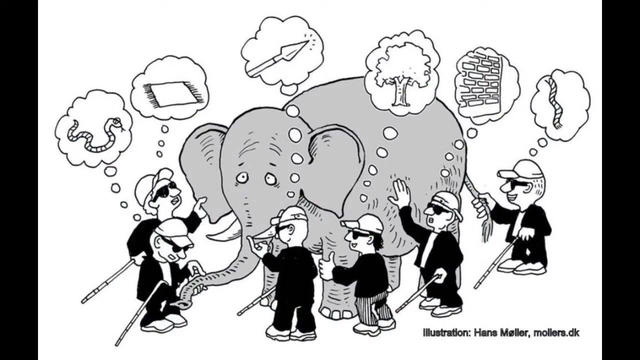 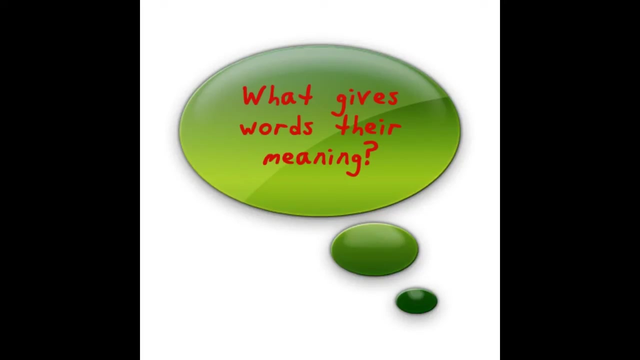 Without a model or an illustration to present the thing as we assume it really exists, descriptions are necessarily ambiguous. The only objective, clear and consistent referent for language and descriptions and any concept in conceivable possibility is meaningful when referring to an object. 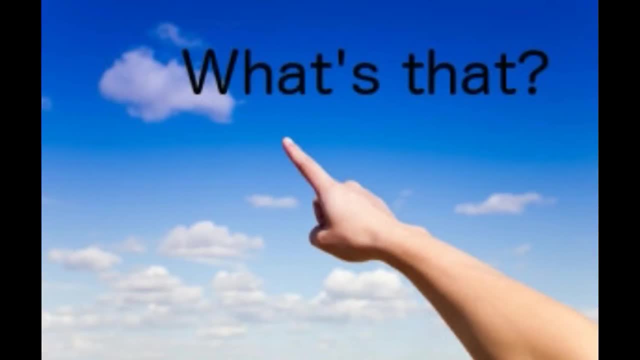 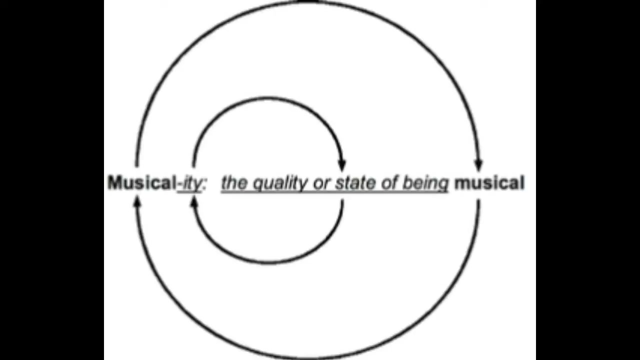 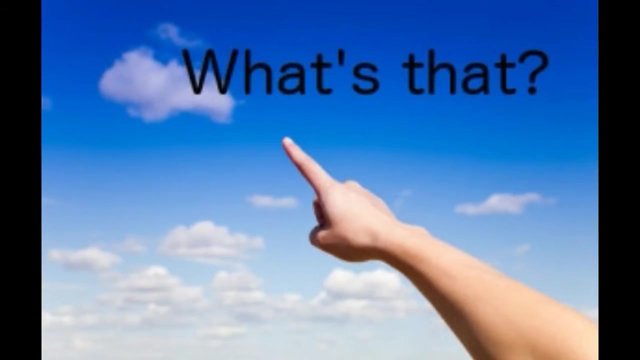 Without a model or an illustration to present the thing as we assume it really exists, descriptions are necessarily ambiguous. The only objective, clear and consistent referent for language and descriptions and any concept in conceivable possibility is meaningful when referring to an object. 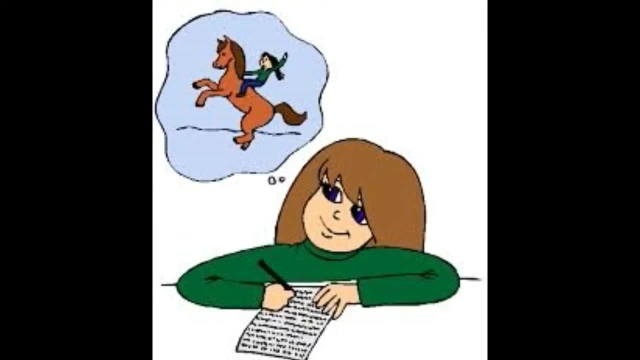 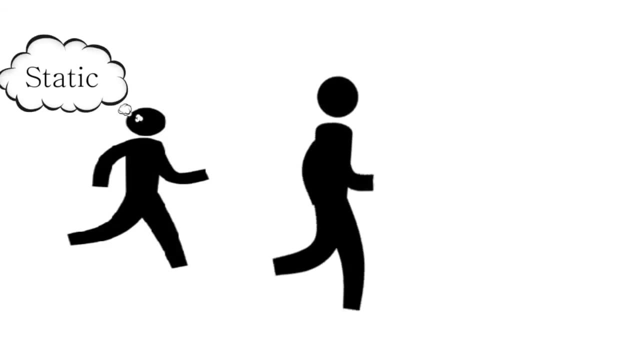 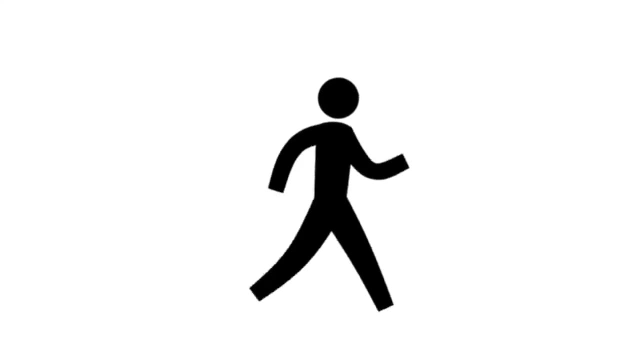 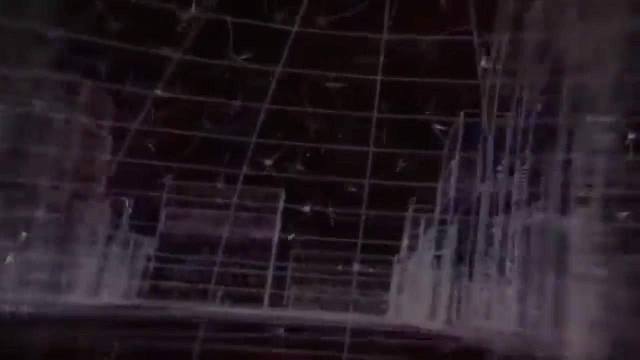 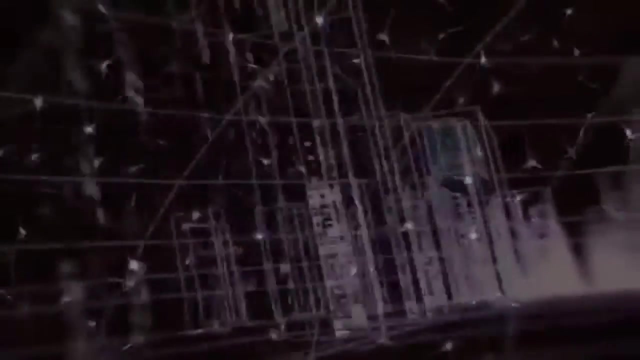 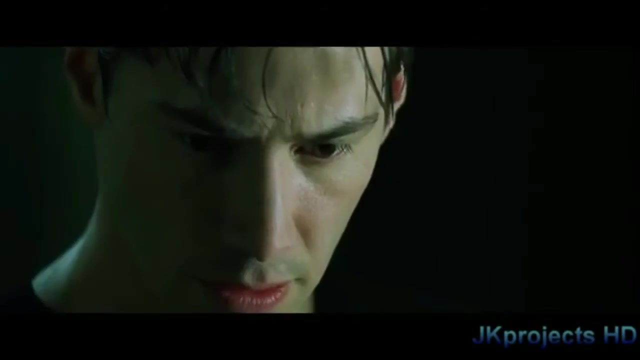 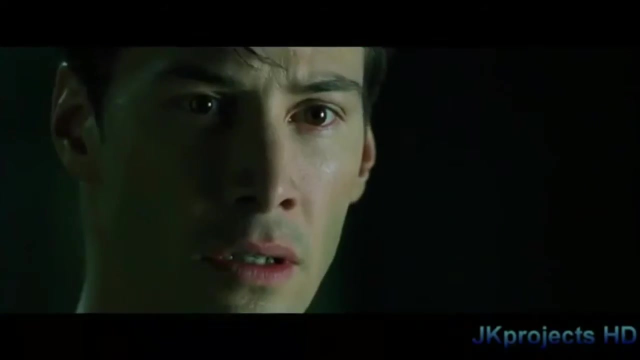 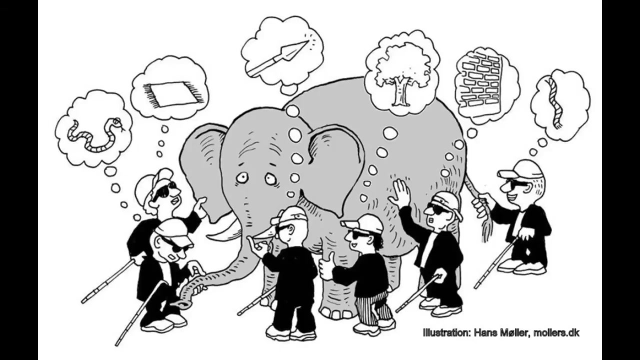 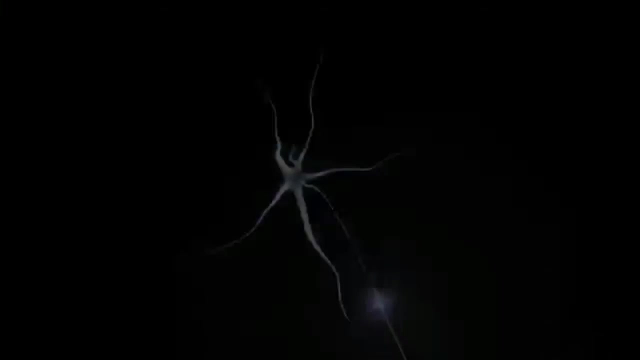 The only objective, clear and consistent referent for language and descriptions, and any concept in conceivable possibility is meaningful when referring to an object. The only objective, clear and consistent referent for language and descriptions, and any concept in conceivable possibility is meaningful when referring to an object. 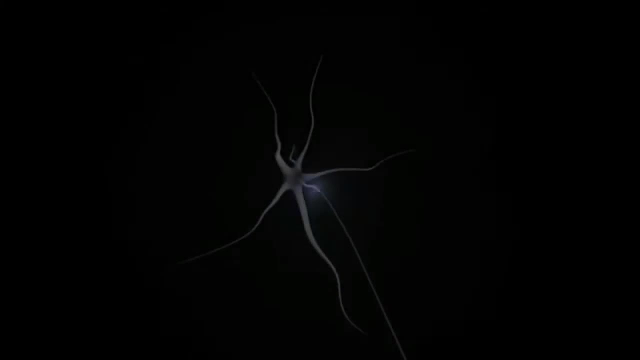 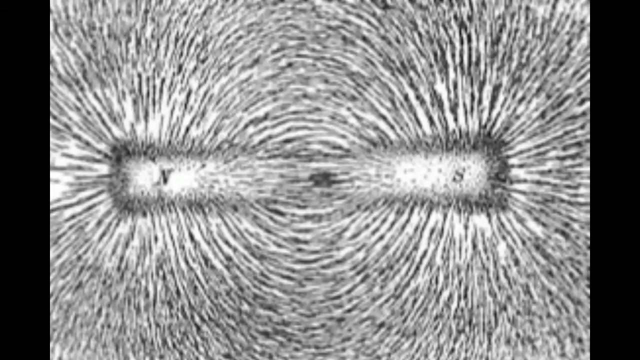 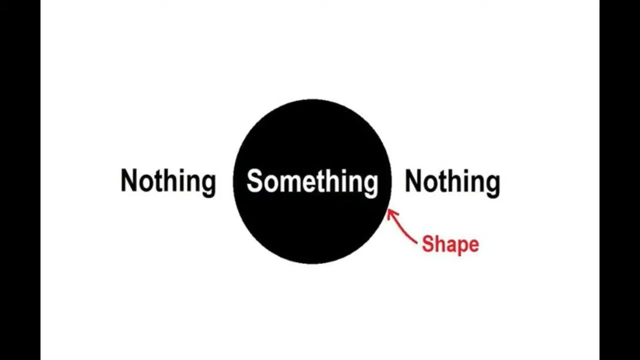 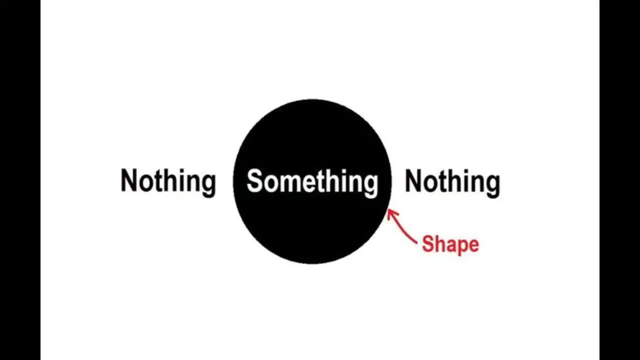 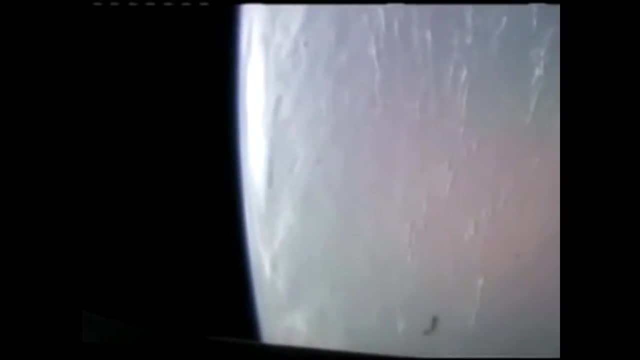 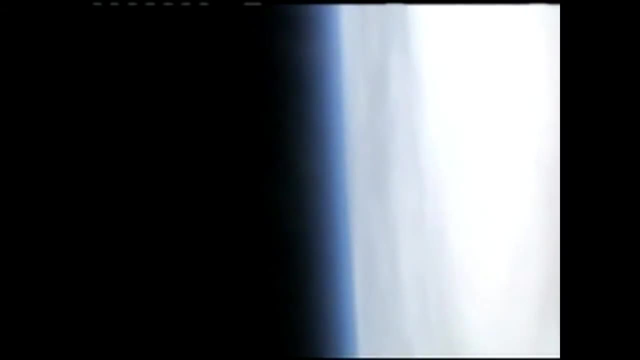 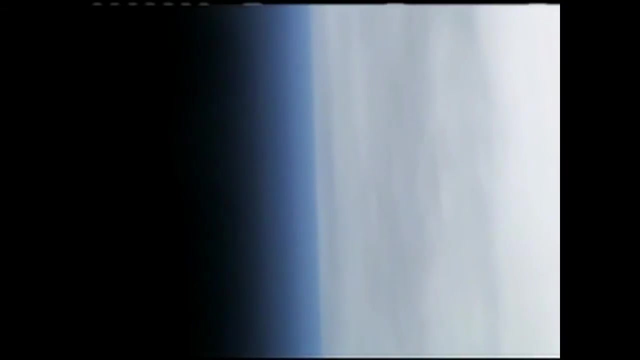 The only objective, clear and consistent referent for language and descriptions, and any concept in conceivable possibility is meaningful when referring to an object. Além from being시다 conundrum, thereím a often asked question. os models步 came member. 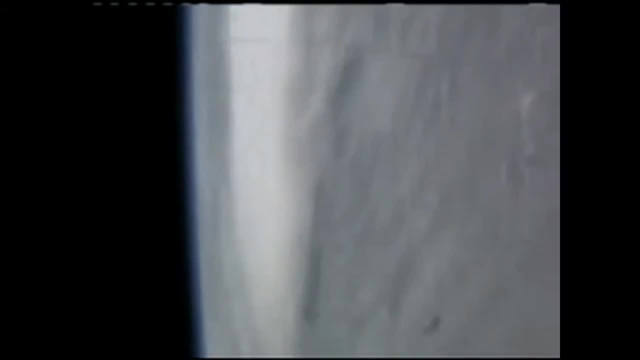 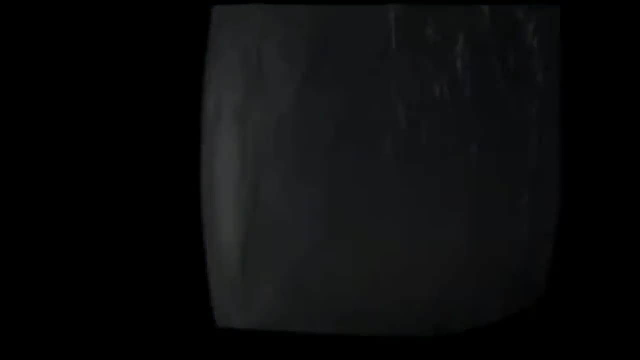 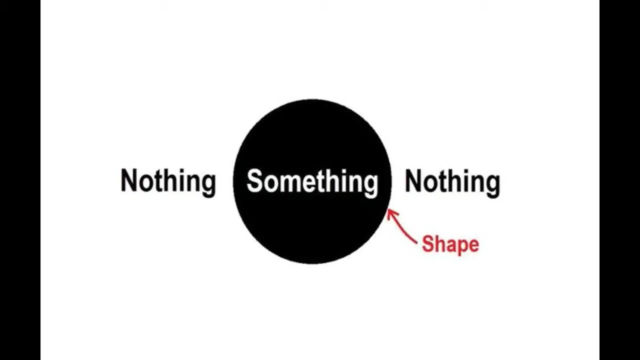 and performs actions. in reality, Form is the intrinsic property of all objects, which allows us to visualize them, no matter how small or big, or far away or invisible they are to our eyes. This is the universal attribute of all things in existence that allows us to think, to comprehend. 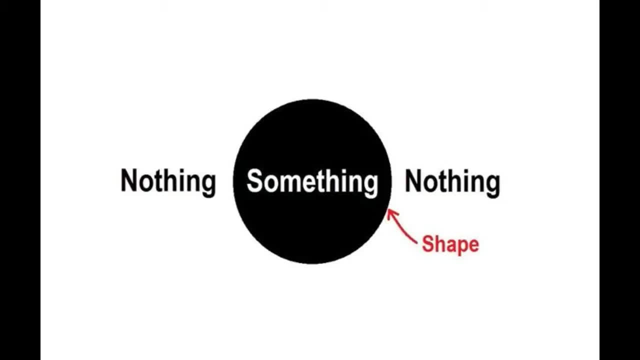 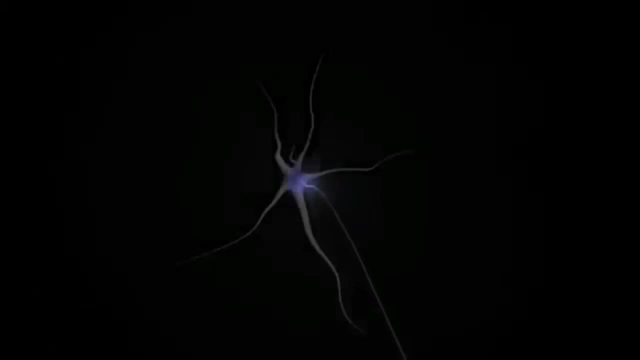 to cognate and to know. Every conceivable word in any language refers either to a form itself or a relationship between forms. Language allows us to think without fully visualizing, but it is only a shortcut, The underlying process which occurs during any thought, any idea, any conception, explanation. 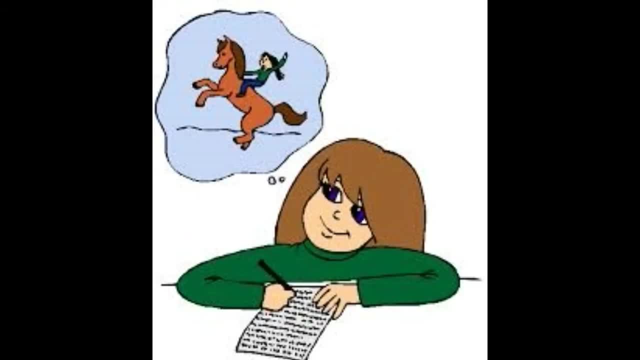 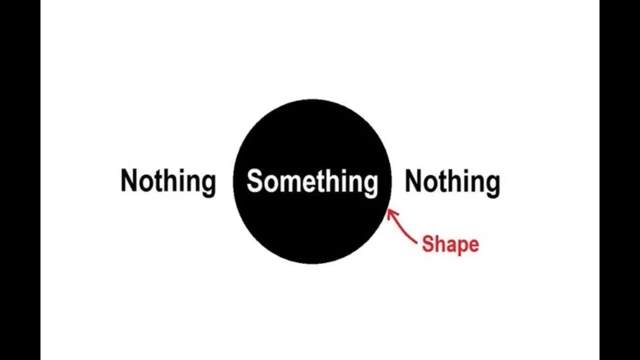 or description is visualization. Without forms to imagine and relate to each other, you literally have nothing. Any statement, description or explanation without ultimate reference to a form or forms is meaningless. The greatest breakthroughs in science have always been new movies of phenomenon to watch. 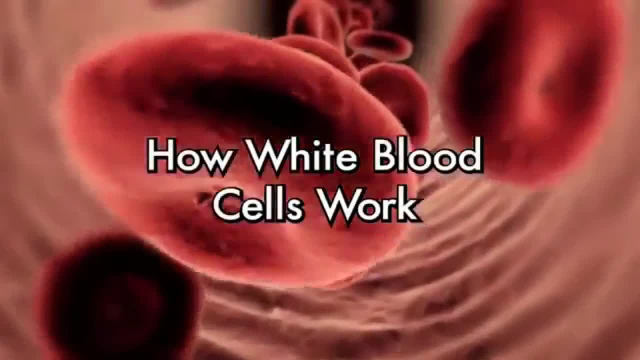 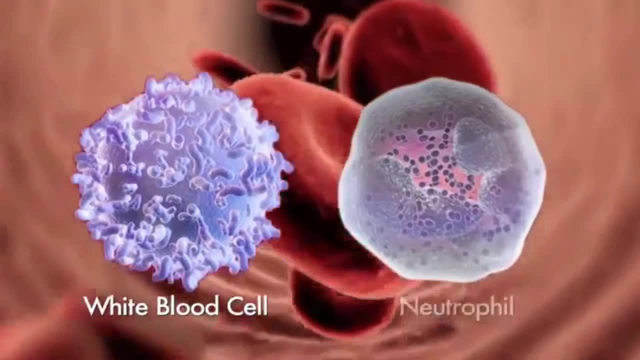 with the objects involved being modeled in full form and detail. Germ theory, for one, is an example of how visualizing the relationships between human cells and bacteria causes us to think. Germ theory, for one, is an example of how visualizing the relationships between human cells and bacteria causes us to think. 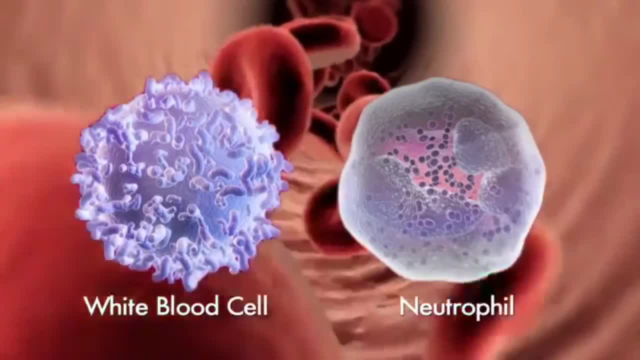 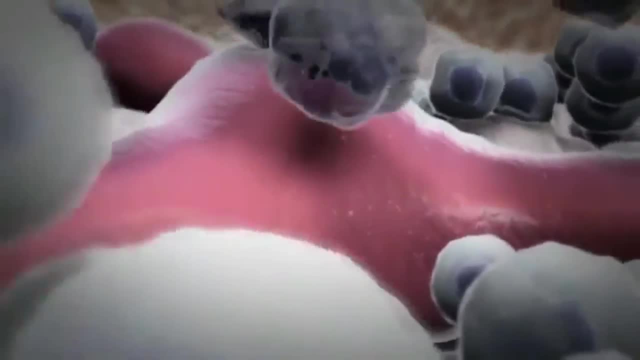 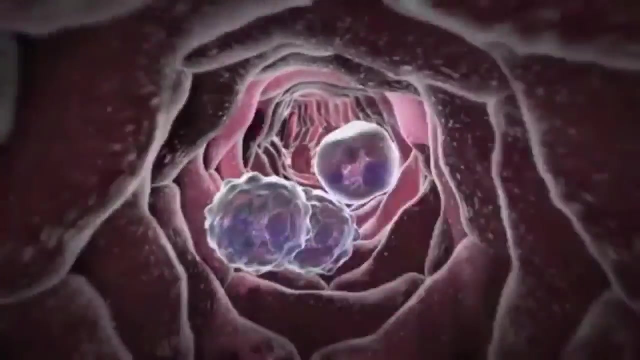 We conceptually shrink down to the size of the cell and imagine every line, curve and detail of its architecture to understand how it works. That is the scientific method. However, during the twentieth century, science has completely rejected these rational routes. However, during the twentieth century, science has completely rejected these rational routes. 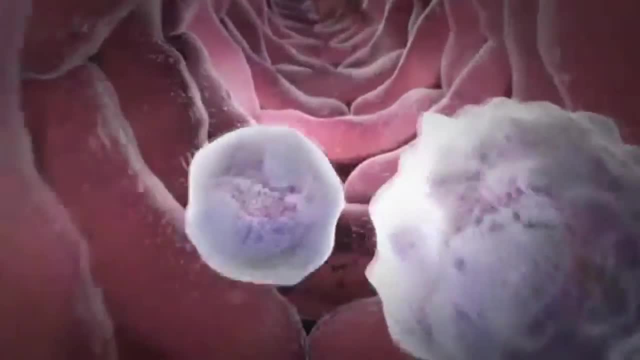 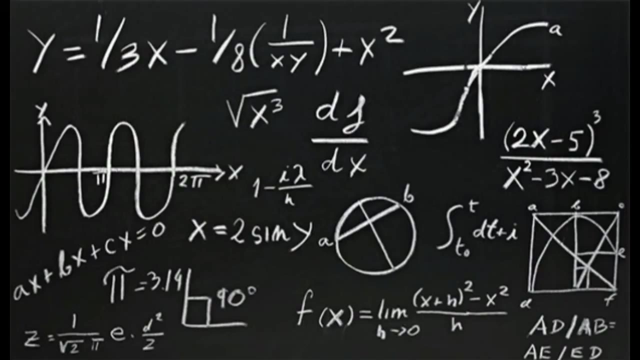 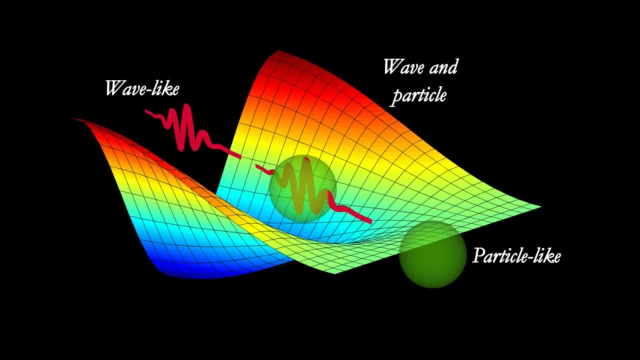 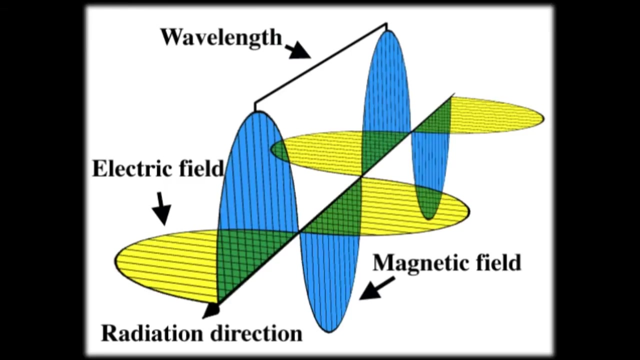 They no longer seek a visualization of any physical phenomena, because they have equated their descriptions themselves with the referent of those descriptions, of those descriptions. They describe the behavior of light, for instance, as waving, and then they convert that description, that verb, into the object itself, The underlying reality of phenomenon. 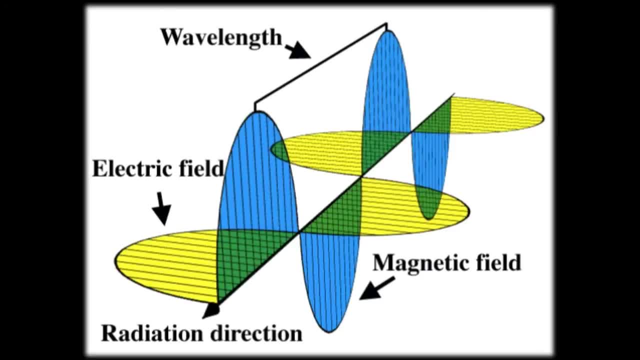 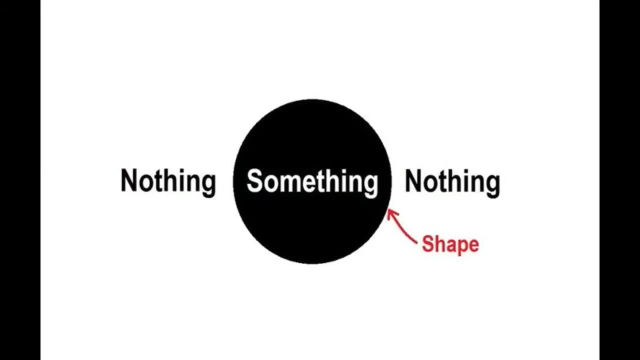 is made up of abstract concepts. to the modern scientist, They have converted all objects into concepts, forgetting that concepts necessarily refer to a relationship between objects. Any concept necessarily invokes objects. So they have created a world full of formless objects and in doing so they have disconnected their theories and descriptions from reality, The underlying 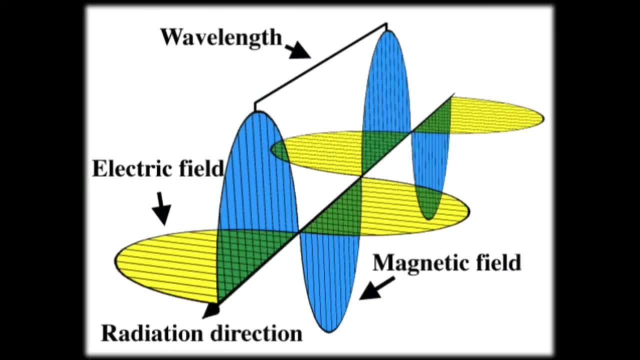 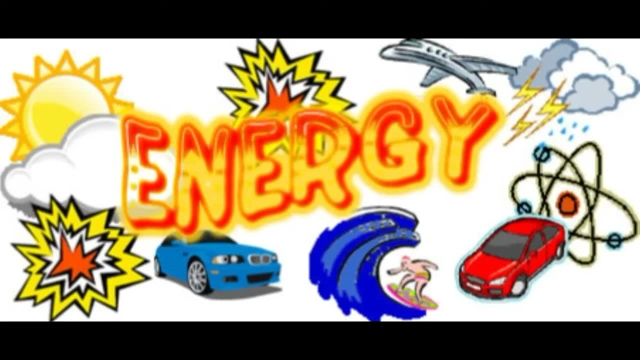 mechanisms that they allege to be responsible for mediating phenomena such as waves, fields, charges, anything are the same. They have created a world full of formless objects and, in doing so, energy etc. are ultimately abstract concepts. They have reduced the subject matter of their 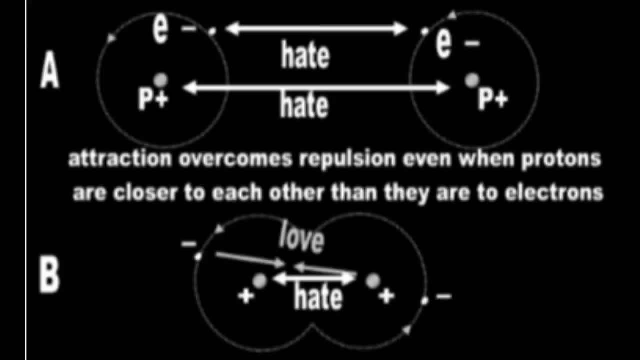 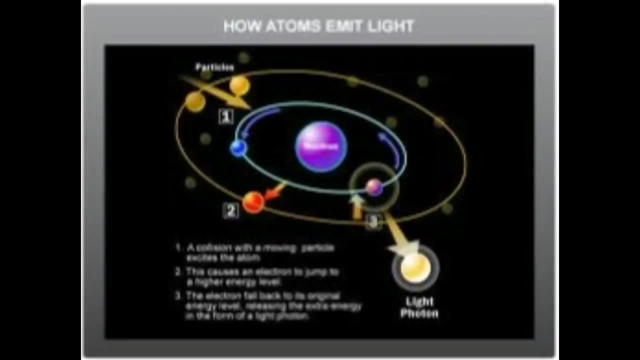 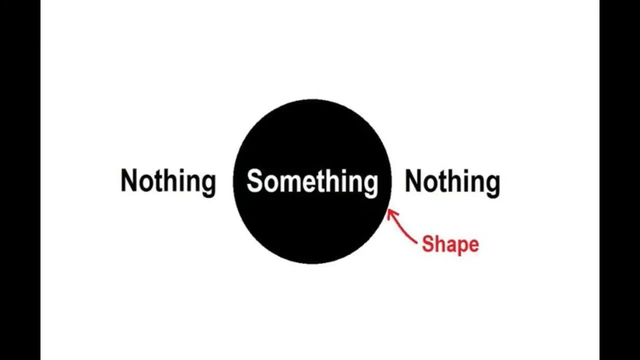 discussion to absolutely nothing at all. By converting their descriptions of the objects into the objects themselves, without presenting an objective model of the forms involved, they have missed the point of science and ultimately divorced themselves from the physical reality of the situation, that is. 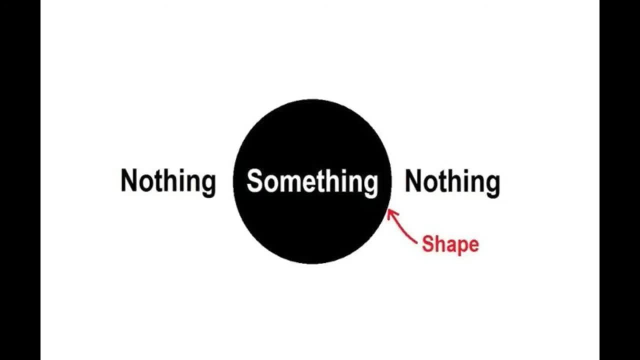 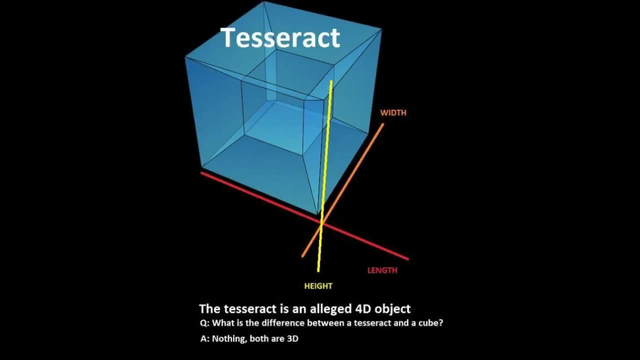 of the object. In total, these, who have been temporarily used as participants, have become contacts with the current objects and relations. Without anything to visualize, without objective models. modern scientists have reverted to religiously studying nothing at all. However, many scientists will tell you straight to your face that there are some objects that cannot be visualized at all. They will refer to objects proposed, objects like spacetime, which they say is four-dimensional and therefore have this. 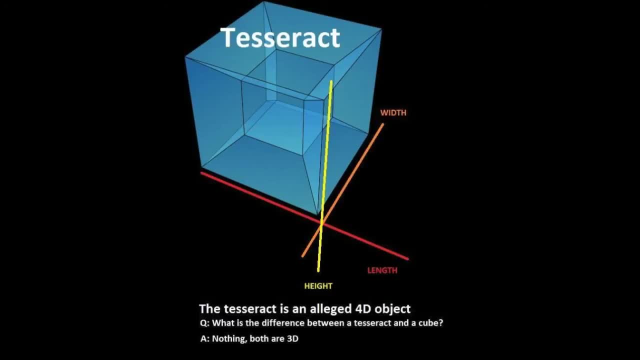 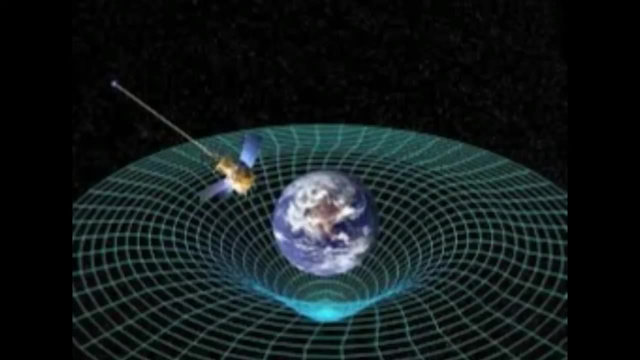 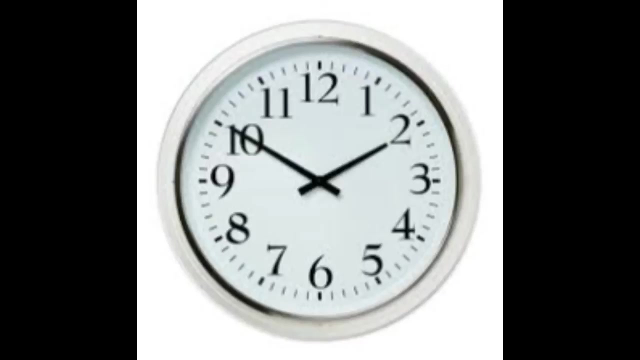 like space-time, which they say is four-dimensional and therefore cannot be visualized or modeled in our petty three-dimensional world. However, it's an irrational belief to think that there are four-dimensional objects. The fourth dimension that they add is time. However, in physics, there are only three. 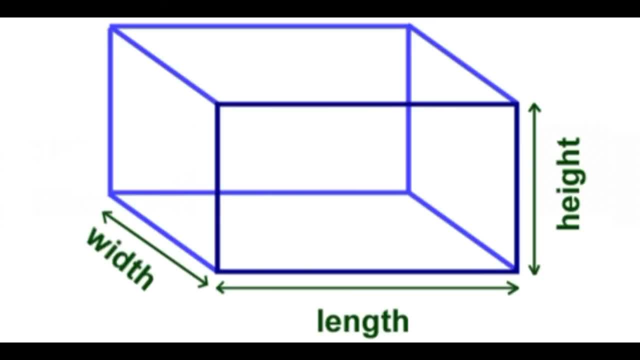 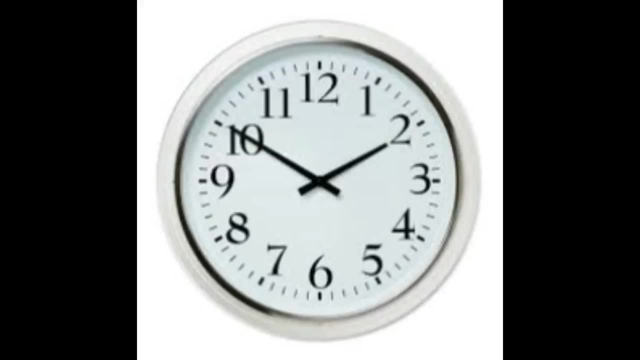 dimensions: length, width and height, since the term dimension, by definition, refers to an object's architecture and orientation. Time refers to neither direction nor an object's architecture and has absolutely nothing to do with the shape of an object. So 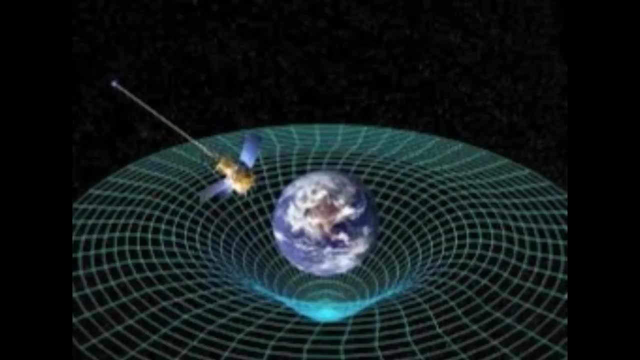 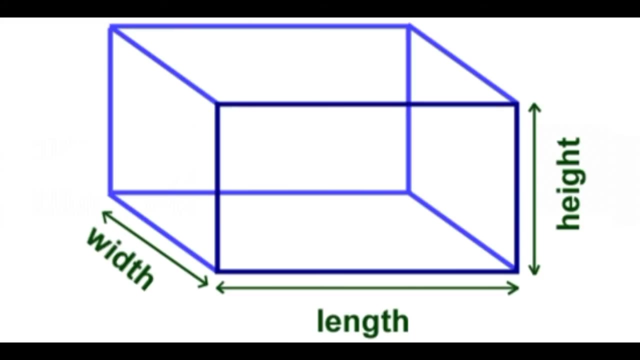 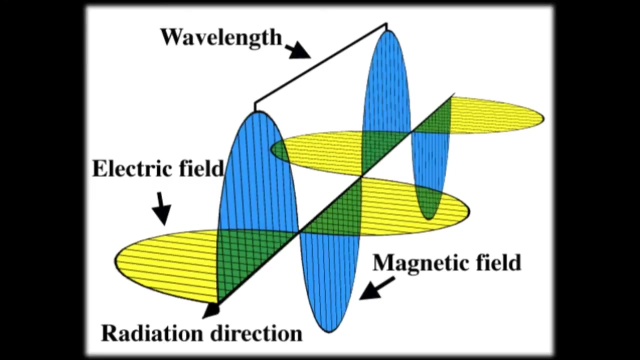 to say that an object is four-dimensional and therefore you cannot visualize it is an irrational belief. It's based on a false misconception of dimensions. They are trapped in a formless, platonic realm of abstract concepts without mediation by physical forms, and yet they still convert these abstract concepts into. 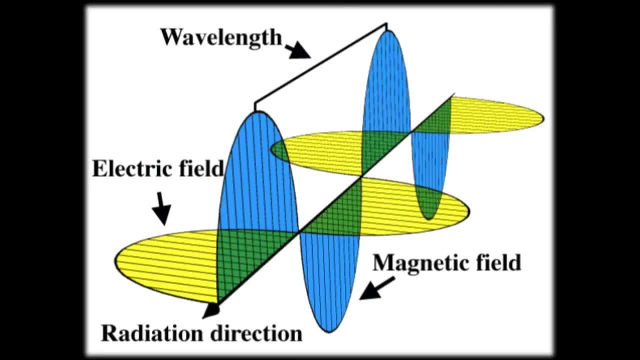 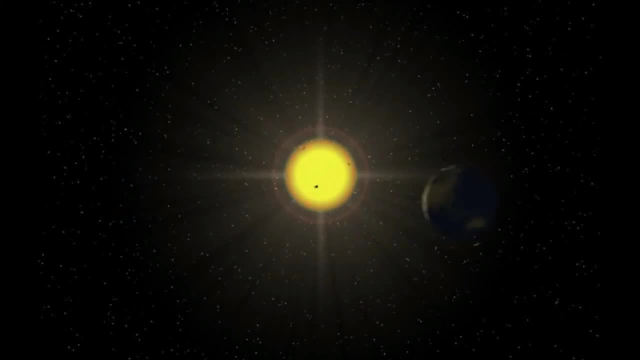 reified avatars or emoticons, such as a loving version of the concept of love, which can be converted into a heart. The wave of motion of an invisible object can become A wave. The action at a distance named gravity and magnetism occurs in a certain area around an object, so they 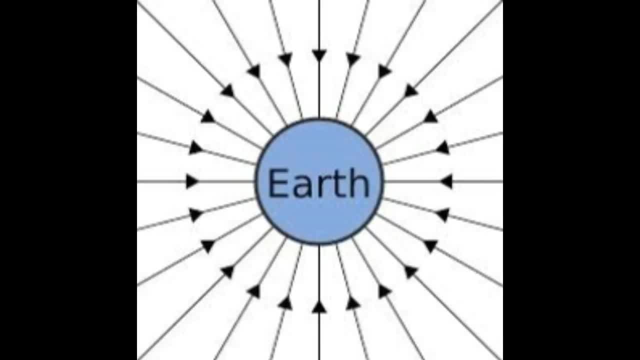 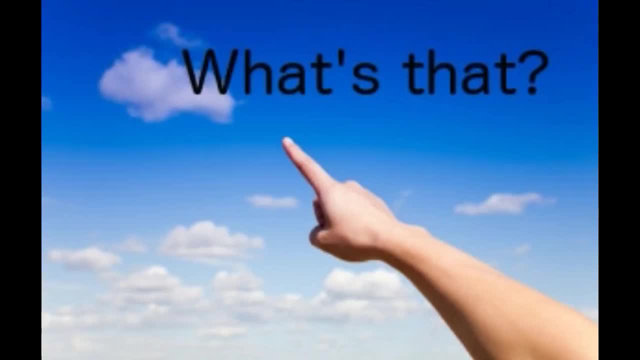 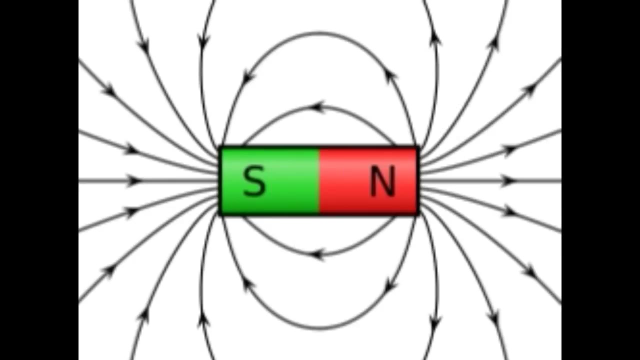 convert that area into the mechanism itself. They are stuck on descriptions without physical forms to reference objectively and, even worse, without it all. Even if this is not worse. they've converted those abstract descriptions into the objects themselves and then try.